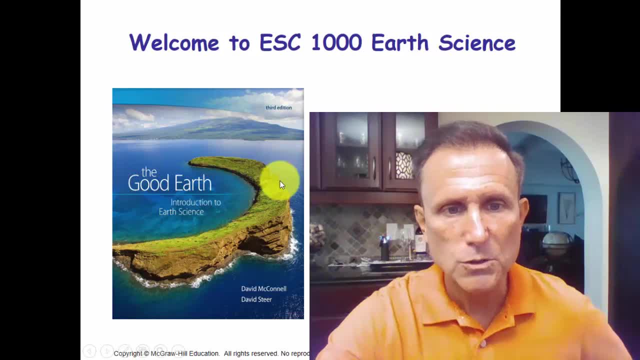 science, and one of the things we're going to talk about will be shield volcanoes And then this little crater that's out here in the ocean, the Pacific Ocean. actually, part of this volcanic system is the Molokini Crater, And it's a little crater that's out here in the Pacific Ocean. 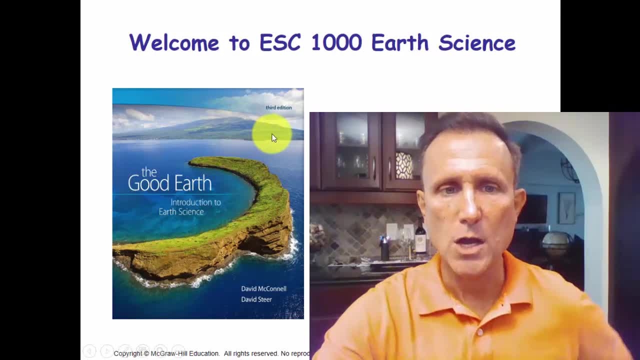 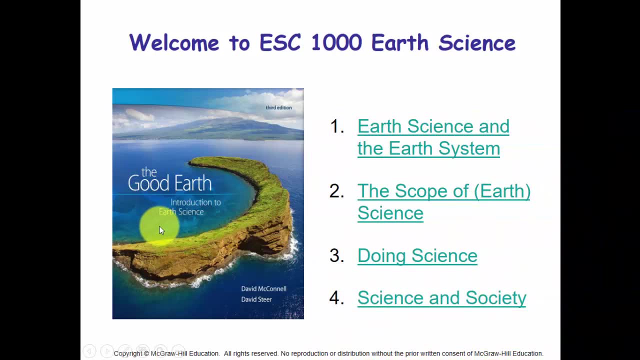 This is a cinder cone that popped up on the side of this shield volcano at a previous time, Now a beautiful spot for diving in a marine sanctuary. So we're going to talk about why the Earth is the way it is and how it got that way. And it's always better to know, and that's why Earth science is. 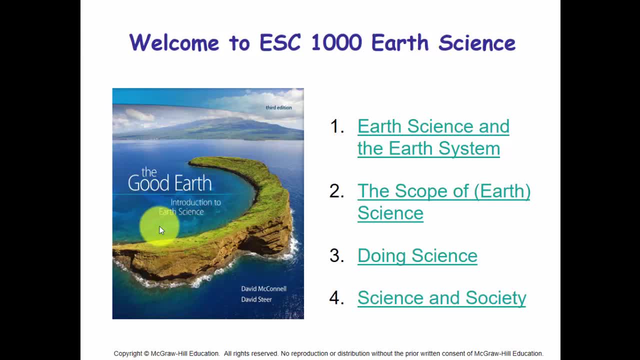 such a great thing to study. So this is an introduction to Earth science. This is chapter one. We're going to talk about Earth science and Earth systems, the scope of Earth science, what it means to do science, to do good science or maybe to do bad science, and then where scientists fit. 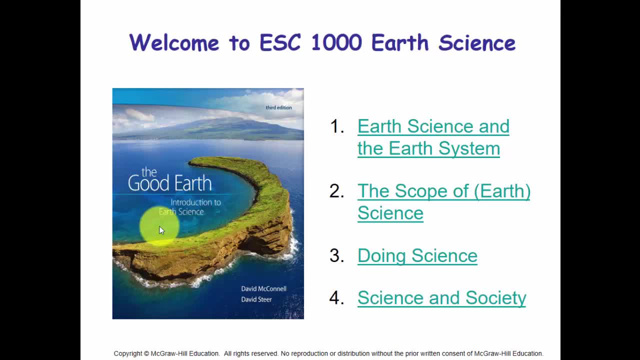 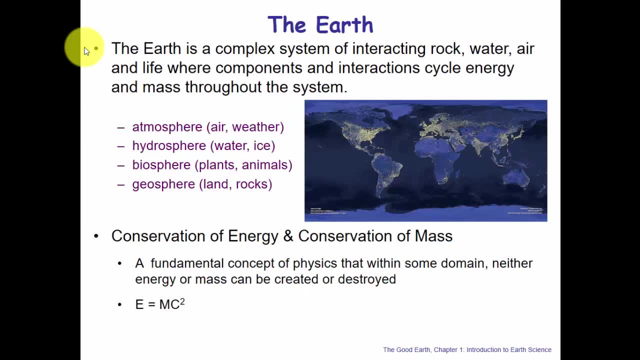 into society. This is a typical beginning of any introductory science class, And then we're going to jump into what's happening with the Earth. Our odyssey, that is, the study of Earth science, begins with the understanding that the Earth is a complex system of interacting rock. 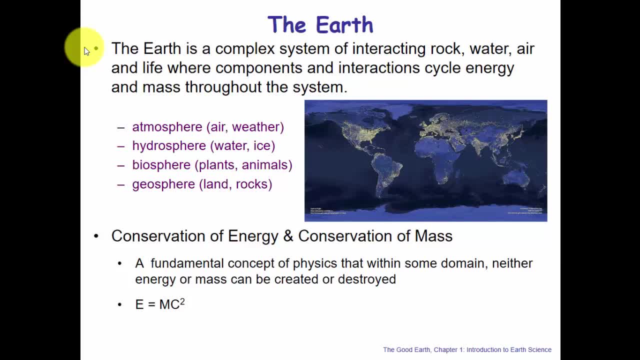 water, air and life, where components and interactions of these four systems cycle energy and mass throughout the whole system, The four systems, of course, being the atmosphere, the air and the weather, the hydrosphere, the water and the ice, the biosphere, the plants. 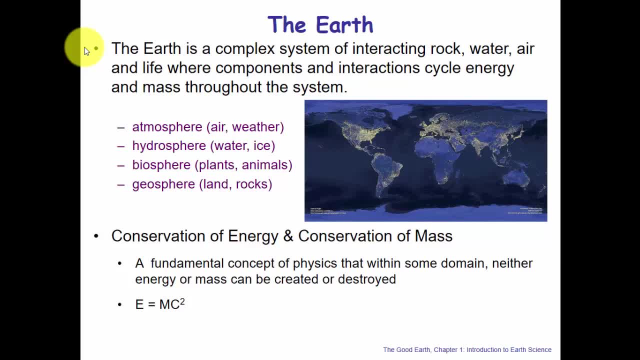 and the animals, and the geosphere, the land and the rocks. Now, this cycling of energy, of mass, refers to the conservation of energy and the conservation of mass. This is the fundamental concept of physics. that says, within some domain, neither energy or mass can be created or destroyed. 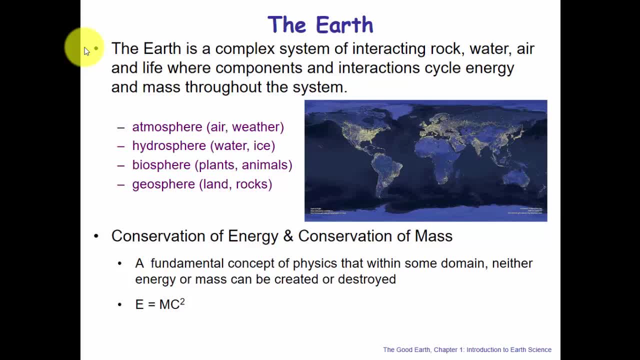 but they can be converted from one to the other, which is where we get the basic formula: E equals mc squared. Energy equals mass times, the speed of light squared. And the speed of light squared is a constant, and so essentially telling us that energy is equal to mass, or energy and mass. 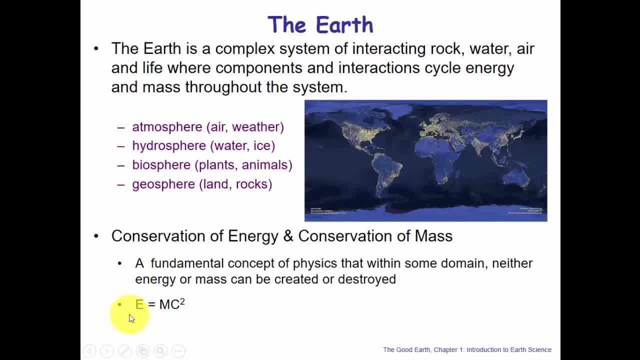 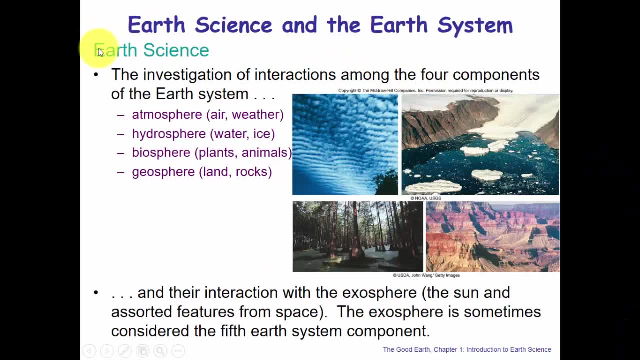 cannot be created or destroyed, but can be cycled back and forth from one to the other: Earth science and the Earth system. We know that Earth science is the investigation of interactions among the four components of the Earth system: The atmosphere, the hydrosphere. 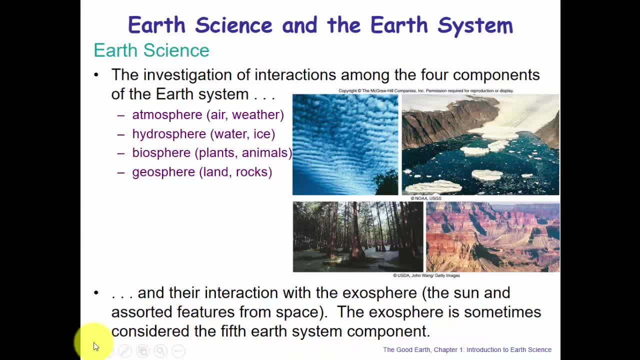 the biosphere and the geosphere, But it also includes the interaction with the exosphere, the sun and the assorted features from space. The exosphere is sometimes considered the fifth Earth system element. So certainly we know the sun interacts with the Earth system, providing us. 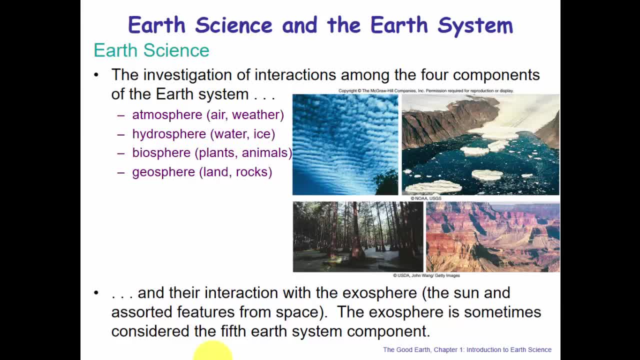 ultimately with all the energy at the Earth system. And the moon also interacts with the Earth system with tidal forces and gravity. So it's not just the four systems, those are the ones we can see in touch here on Earth. There's also the solar system, the solar system, the solar 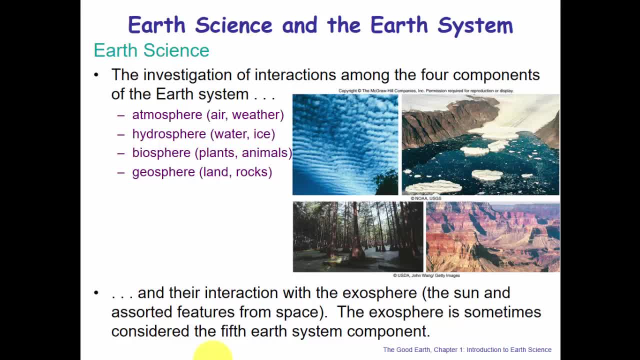 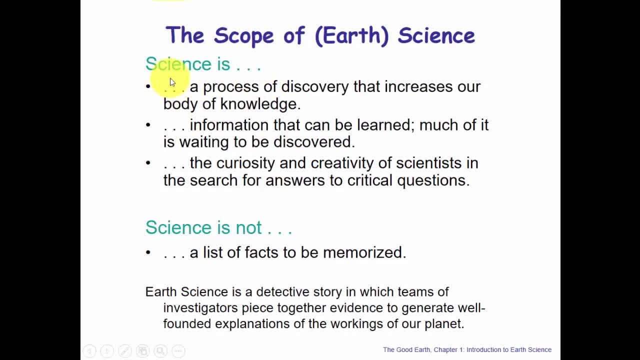 system. Now the fifth system was in space and all around us in space. To understand Earth science, we need to understand what science is at its core And in its essence. science is simply a process of discovery. Now, it's a process of discovery that increases our body of knowledge. Science is 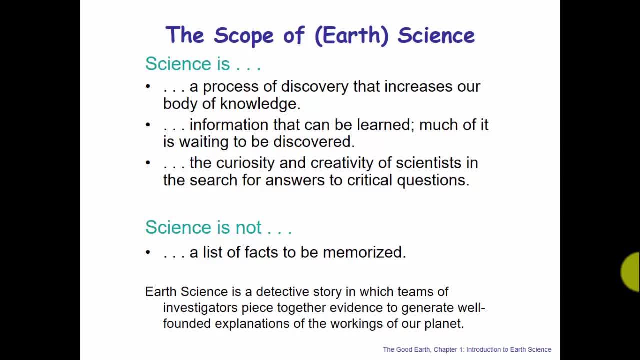 information that can be learned, much of it just waiting to be discovered. Science is also the curiosity and creativity of scientists and their search for information, So it's a process of discovery that increases our body of knowledge. Science is simply a process of discovery. Now. 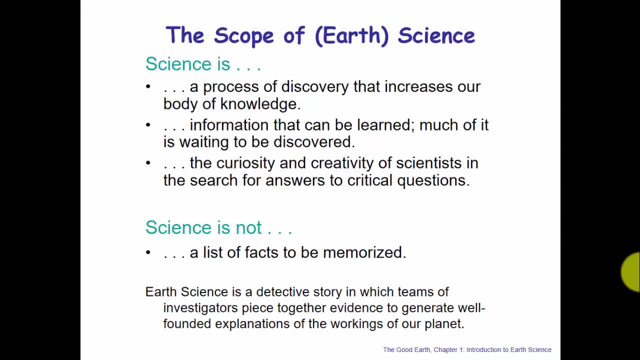 what science is not is a list of facts to be memorized. Earth science is a detective story in which teams of investigators not always even working together, but teams of investigators piece together evidence to generate well-founded explanations of the workings of our planet. And 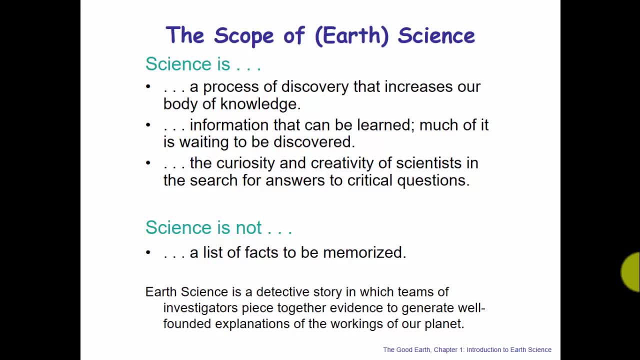 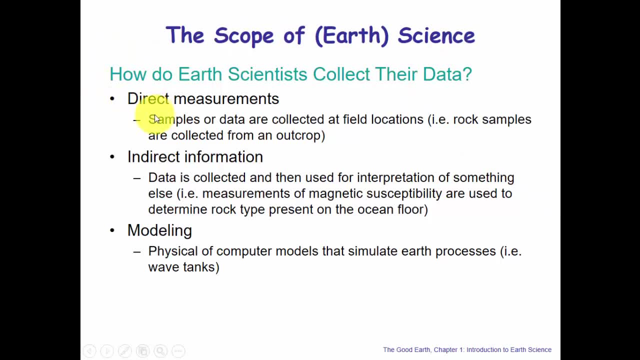 that evidence comes from observations and data. How do Earth scientists collect that data? Well, through direct measurements, Direct information and modeling. And, of course, direct measurements is literally going out there and measuring what's happening on the Earth, in the crust, in a sinkhole: the Grand Canyon. 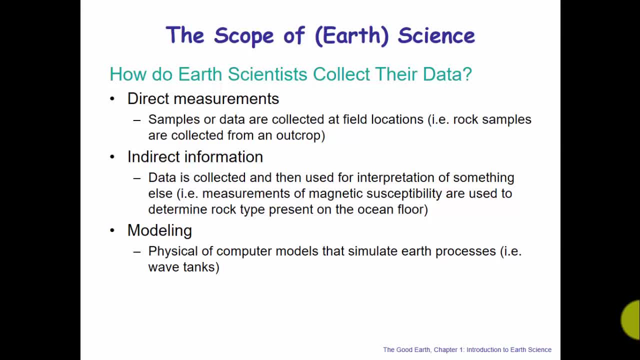 collecting rock samples from an outcrop. Samples are data collected at field locations. Now, indirect information is when data is collected, but then it's used for the interpretation of something else completely. For instance, we collect ice cores- literally long cores of ice. 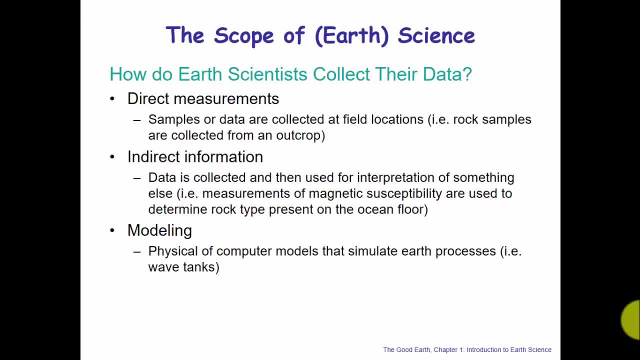 many meters long down into the glacier on top of Antarctica And from those ice cores, by setting that ice and the gas bubbles in that ice, we can interpretate and make interpretations, that is, of other things such as climate in the distant past. So indirect information is collecting data and then using that. 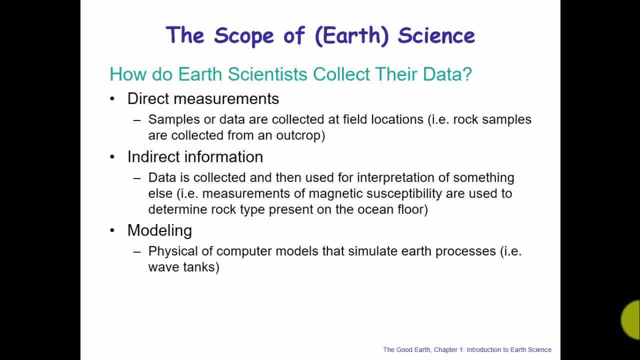 data for the interpretation of something else And, of course, modeling. talk a lot about modeling. We talk about hurricanes and weather models, hurricane models. Modeling is also the creation of physical models, like a wave tank In which we can study how waves interact and how computer models and physical models together. 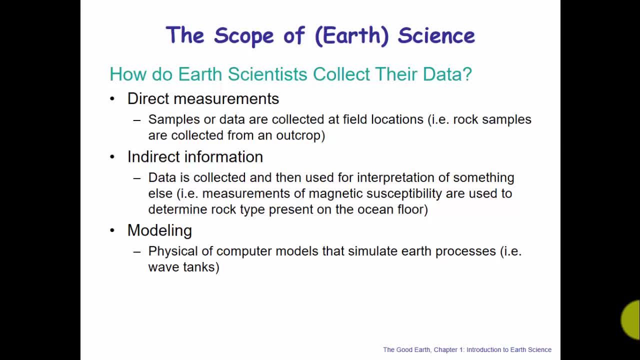 maybe to determine how the Gulf of Mexico would handle a hurricane- not the winds and the rain, but the storm surge- and how large bodies of water deal with waves being pushed across them. We use physical wave tanks and computer models to collect that data. 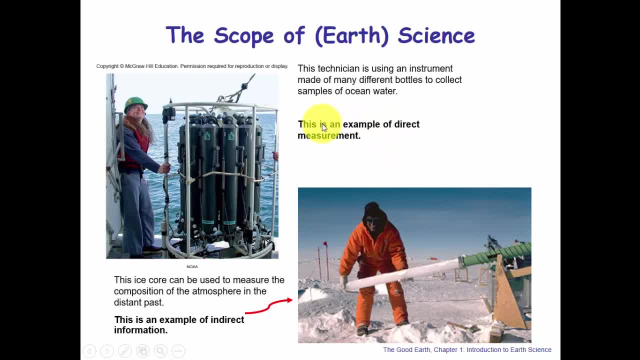 So here are some examples of that data collection. In the upper left, technician is collecting bottles of water from the ocean, samples of ocean water for lots of water. That's a different research. That's an example of direct measurement. And there's one of those ice cores. 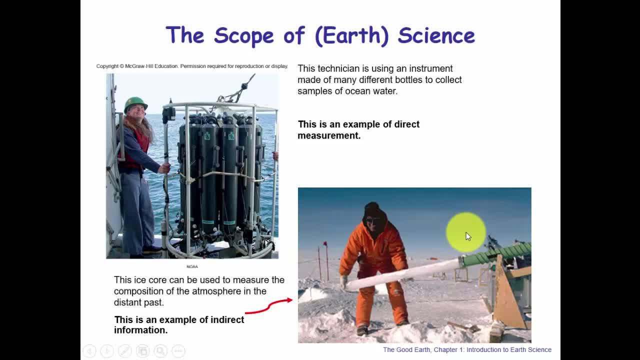 You can see the scientist there in the lower right. Ice core can be used to measure the composition of the atmosphere in the distant past And that's an example of the collection of indirect information. And here is an example of one of those wave pools. 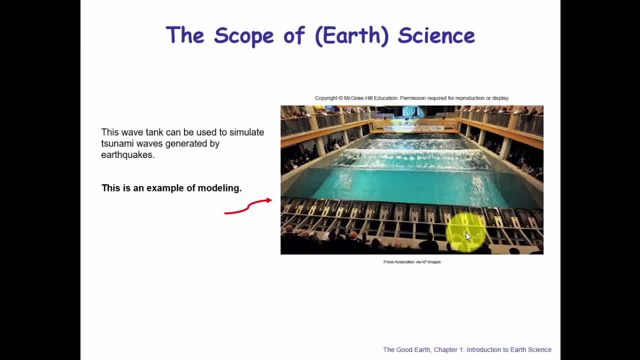 Now look at the left side of this picture. You can see the people. So this gives you an idea of just how large this wave pool actually is, And that is your example of physical modeling, And during the course of this class, we're going to talk a little bit more about that. 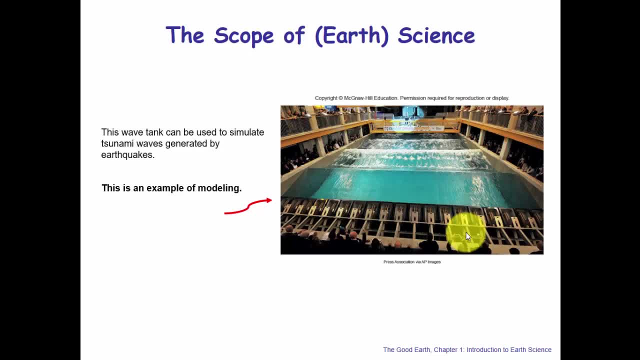 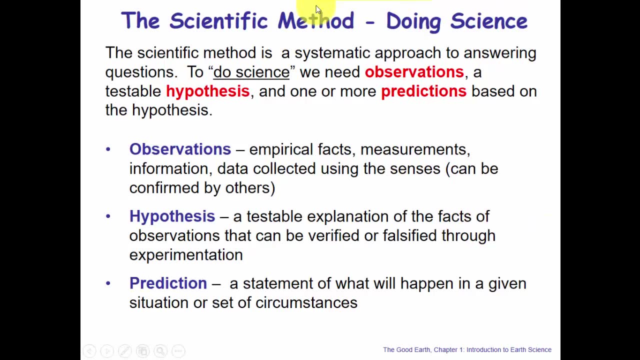 We're also going to take a look at computer models, specifically with weather models. By now, most of you, in one science class or another, have been exposed to the idea of the scientific method, And the scientific method is that systematic approach to answering questions. 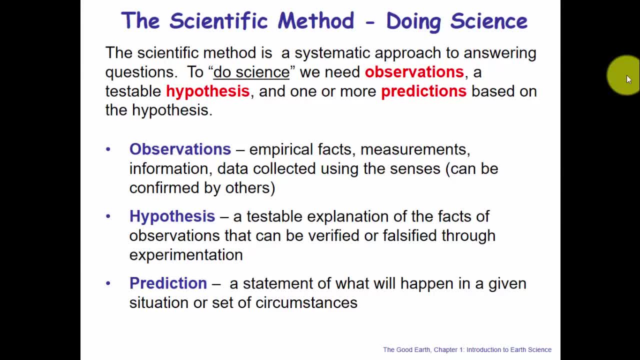 And to do this we need observations, a testable hypothesis and one or more predictions based on that hypothesis. The observations, of course, empirical facts, Measurements, information, data collected using the senses, Something that can be confirmed by others, whether it's actual observations in the field or observations in data based on models. 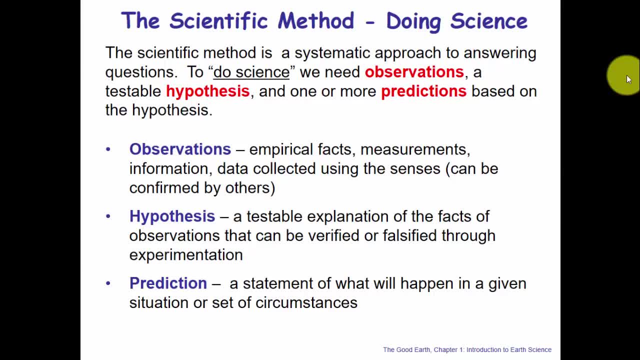 That hypothesis, a testable explanation of the facts, of the observations that can also be verified or falsified through experimentation. So it's an explanation of those facts, of that data that you measured or observed, But it's a testable explanation that can be verified or, in some cases, falsified through experimentation. 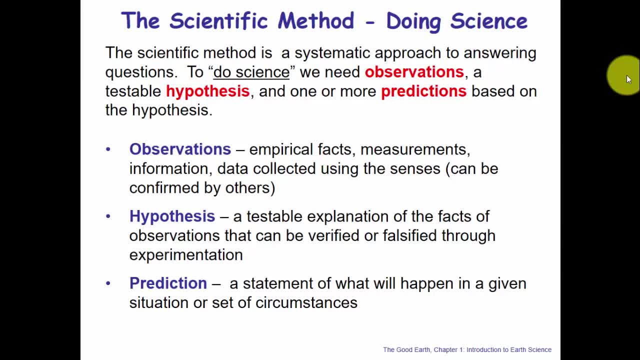 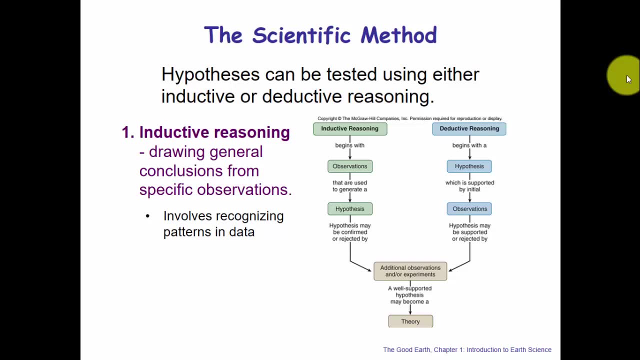 And then a prediction. With all this, you can make a prediction, a statement of what will happen in a given situation or set of circumstances, based on those hypotheses and observations. The hypothesis or that explanation of data or observations can be tested using either inductive or deductive reasoning. 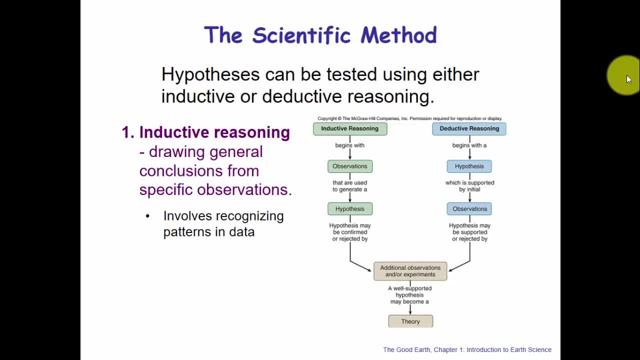 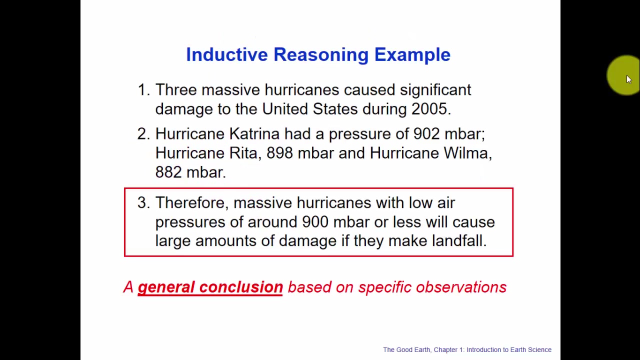 Remember, a hypothesis has to be able to be tested by others in order for it to be verified. So what is inductive reasoning? Drawing general conclusions from specific observations? So it involves recognizing patterns in the data. You're drawing general conclusions from specific observations. 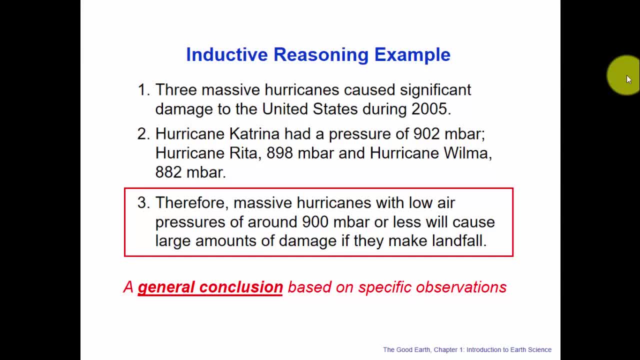 Here is an example of inductive reasoning. Number one: Three massive hurricanes caused significant damage to the United States during 2005.. Number two: Hurricane Katrina had a pressure of 902 millibars. Hurricane Rita: 898 millibars. 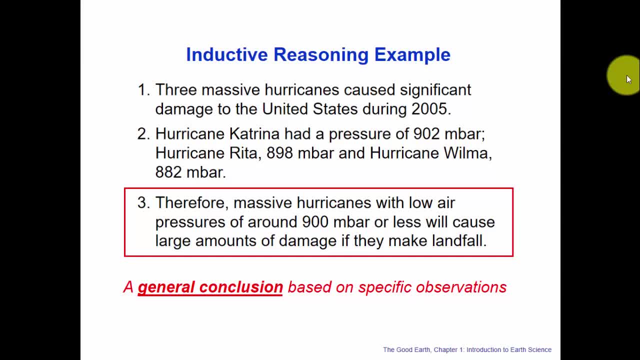 And Hurricane Wilma 882 millibars. The inductive reasoning would allow you to draw the general conclusion, based on specific observations, that massive hurricanes with low air pressure around 900 millibars or less will cause large amounts of damage if they make landfall. 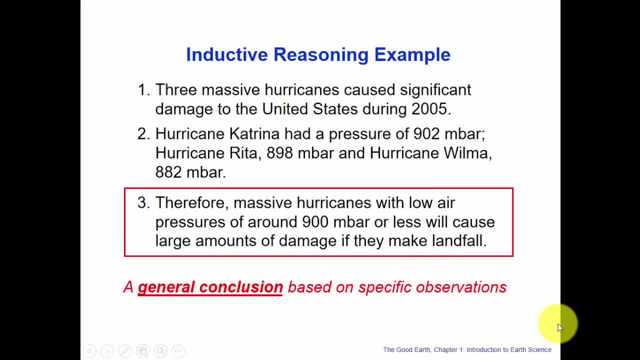 Knowing that those three hurricanes with central pressures of around 900 millibars cause massive damage can allow you to make that general conclusion that massive hurricanes with central pressures of about 900 millibars will cause large amounts of damage if they make landfall. 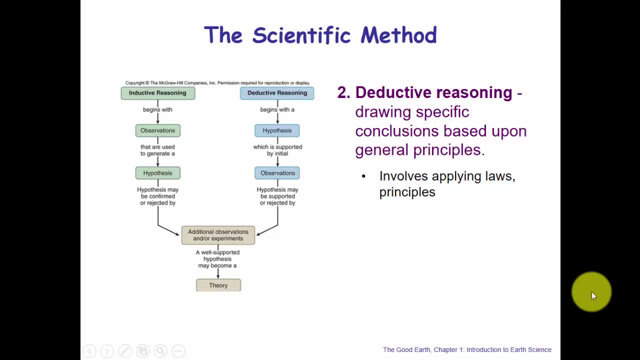 The other methodology that can be used to test the hypothesis is deductive reasoning. Now, in deductive reasoning, you are drawing specific conclusions based on general principles. This involves applying laws and principles to look at the data or the observations and then to come up with specific conclusions about that data or those observations. 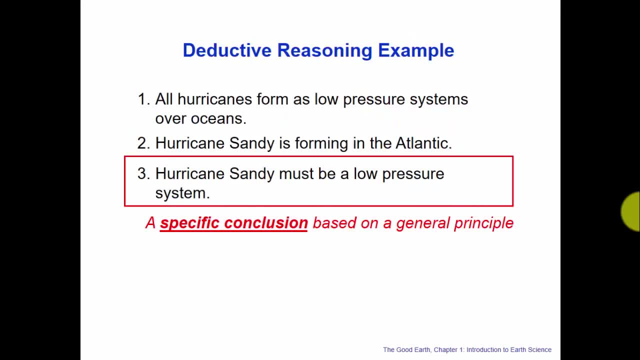 Here is an example of deductive reasoning from the world of tropical meteorology, again. Number one: All hurricanes form as low pressure systems over oceans. Number two: Hurricane Sandy is forming in the Atlantic. So the deductive reasoning or the specific conclusion based on a general principle is: Hurricane Sandy must be a low pressure system. 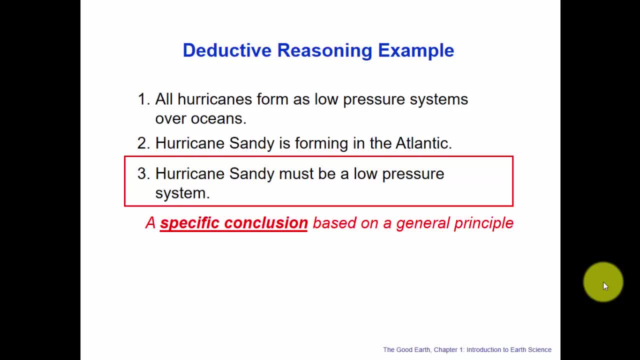 If all hurricanes form as low pressure systems over oceans and Hurricane Sandy is forming over the Atlantic, which is an ocean, we then know that Hurricane Sandy is also a low pressure system. Using deductive reasoning, we deduce that it must also be a low pressure system. 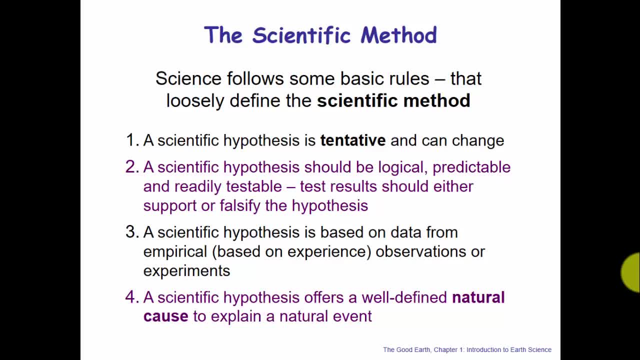 Back to the general notion of the scientific method. The scientific method is something that allows us to do science well, to do good science, And science follows some basic rules that are loosely defined as the scientific method. So a scientific hypothesis is a tentative thing. 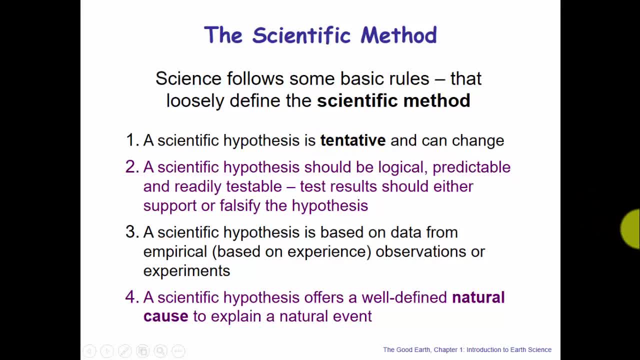 It can be changed. It's something that's not absolute, It's just a hypothesis, And that hypothesis must be able to be either completely or partially changed. A scientific hypothesis should be logical, predictable and readily testable, And test results should either support or falsify the hypothesis. 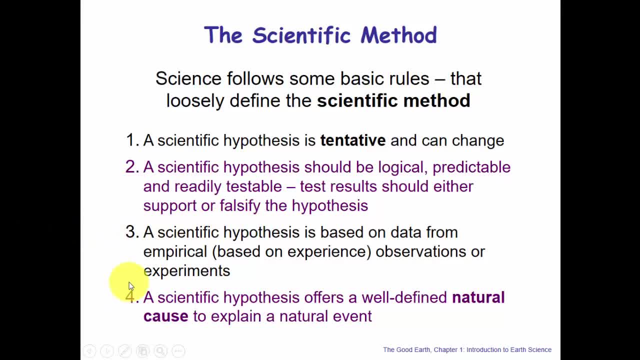 A scientific hypothesis is based on data from empirical, based on experience- something you actually saw, empirical observations or experiments- And a scientific hypothesis offers a well-defined natural cause to explain a natural event. If the hypothesis is saying that volcanoes cause lots more CO2, carbon dioxide to be in the atmosphere, 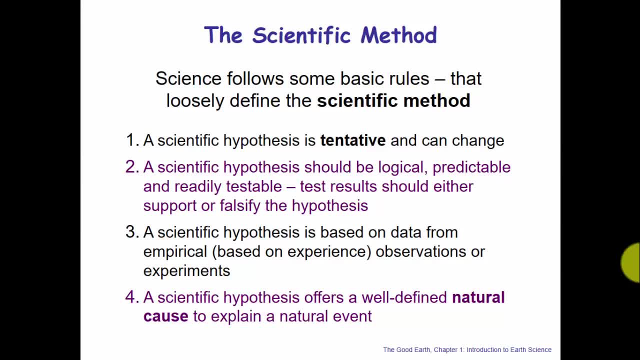 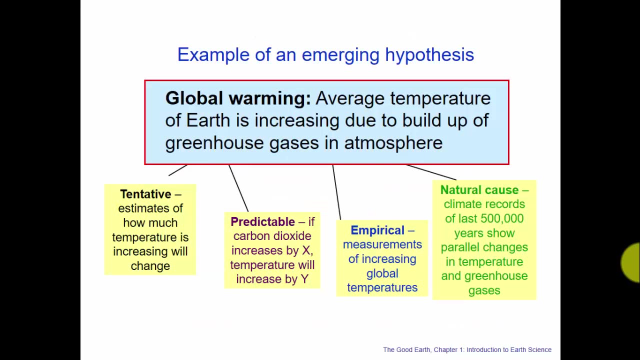 then there has to be a well-defined natural cause that shows how the CO2 gets from the volcano to the atmosphere or how the volcano causes CO2 to be in the atmosphere. There has to be a well-defined natural cause. So here is another example of a hypothesis. 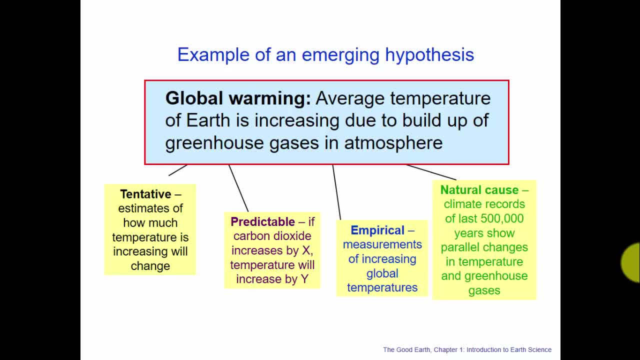 This is an emerging hypothesis and a hypothesis that we hear a lot about in the media today, And we're going to show how this hypothesis has to be tentative, predictable, empirical and also have a natural cause: Global warming. Average temperature of the Earth is increasing due to a buildup of greenhouse gases in the atmosphere. 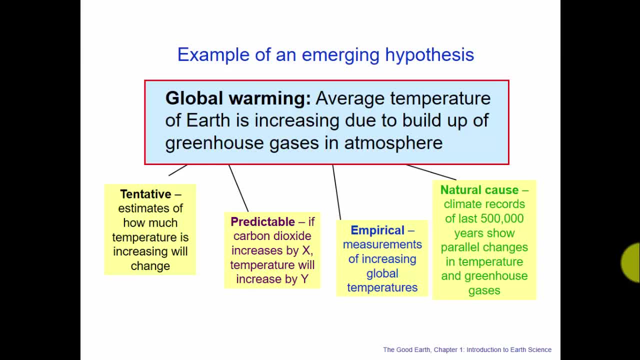 So that's our hypothesis. We look at all the data, we make all these observations and our hypothesis is that global warming is occurring or our hypothesis is that the average temperature of the Earth is increasing due to the buildup of greenhouse gases in the atmosphere. 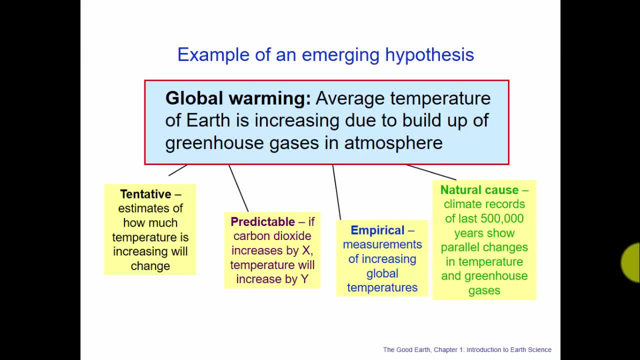 That's the reason why the Earth's temperature is increasing: because of the buildup of greenhouse gases in the atmosphere. Not because the Sun is hotter or the core of the Earth is hotter or there's a second star close by, but the hypothesis is that greenhouse gases in the atmosphere are increasing. 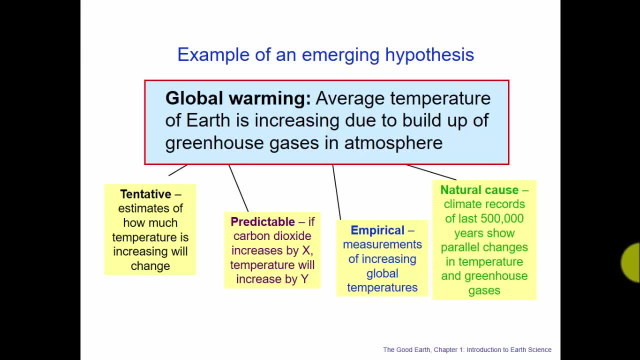 They're building up, The Earth is warming. This hypothesis is tentative. Estimates of how much temperature is increasing will change, meaning. some scientists and some models give us a 2 or 3 degree temperature increase over 50 years. Some give us a 2 or 3 degree temperature increase over 500 years. 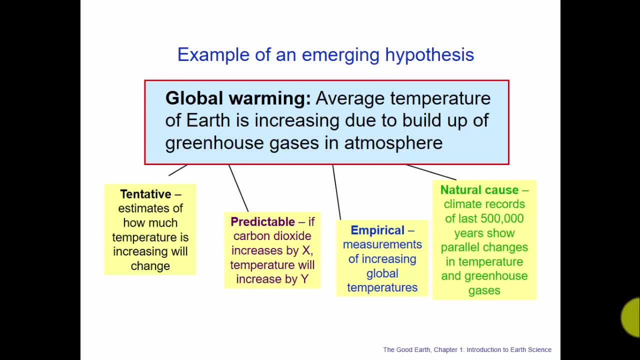 It's also predictable. The prediction is that if greenhouse gases such as carbon dioxide increase by this amount, then temperatures will increase by this amount. It's empirical. We are making measurements of increasing global temperatures. We have a record of global temperatures and we can see an increase there. 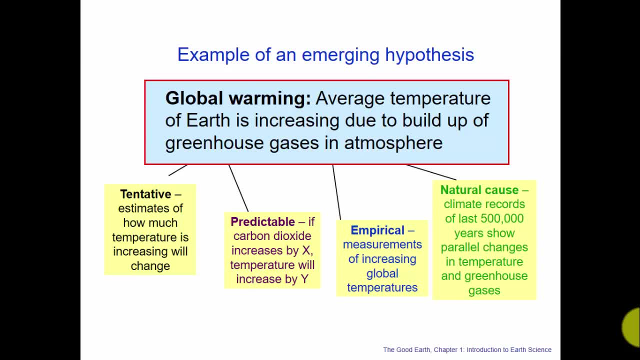 and we also have a record of greenhouse gases in the atmosphere and we can see the similar increase there. So it's an empirical thing. We actually have experience or observations to back this up and we can provide this natural cause. Climate records, literally over 500,000 years, show parallel changes. 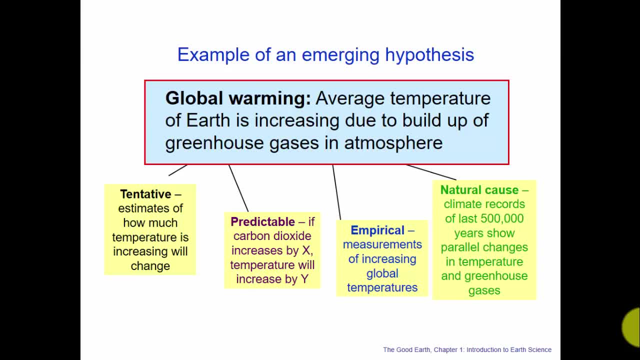 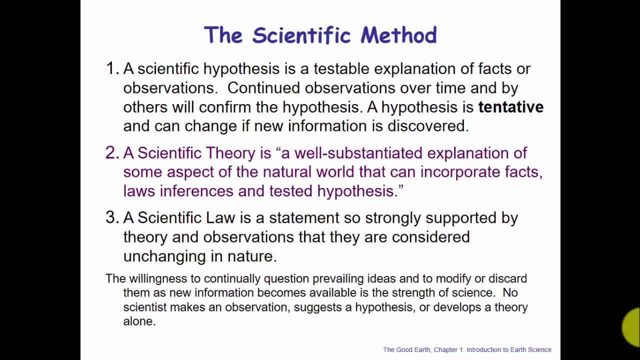 in temperature in greenhouse gases. We can show how there's a natural cause that greenhouse gases increase the Earth's temperature, because greenhouse gases absorb infrared radiation being emitted by the Earth and hold it, and that's the natural cause. So let's clear up the confusion between hypothesis theory and law. 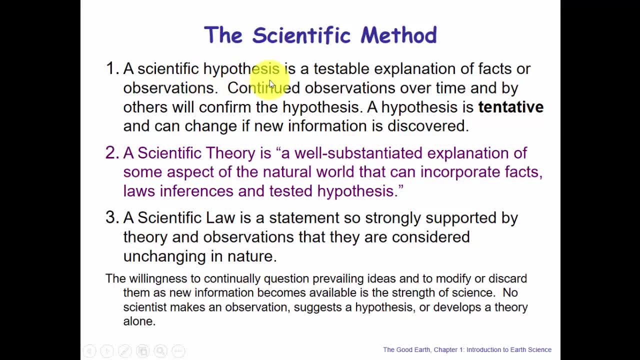 A scientific hypothesis is a testable explanation of facts or observations or data. Okay, That's it, Testable explanation of the facts. You see a bunch of this and you give an explanation of that. Continued observations over time and by others will confirm the hypothesis. 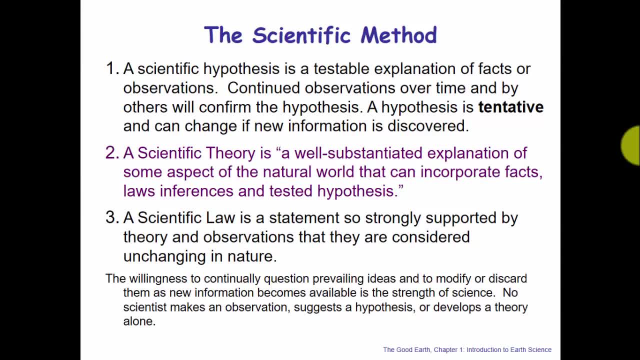 Yeah, we saw a bunch of the same thing, and that confirms your hypothesis. A hypothesis is tentative. It has to be able to change if new information is discovered. Yes, we saw a bunch of the same thing, but we also saw this. 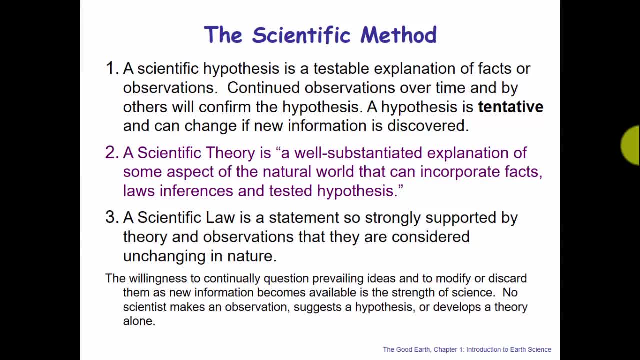 and that slightly changes your explanation. A scientific theory is now a well-substantiated explanation of some aspect of the natural world that can incorporate facts, laws, inferences and tested hypothesis. A theory now is when we basically have an agreement by the lion's share of the scientific community. 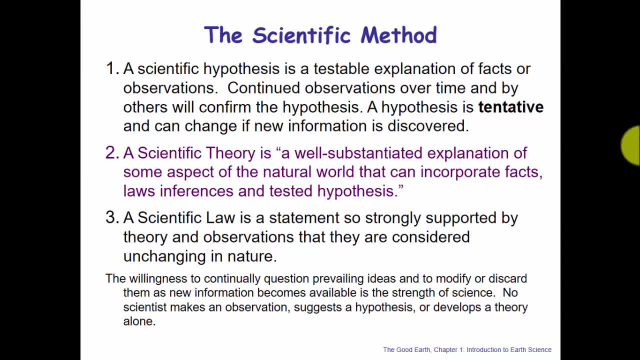 based on the same observations and the same data, that they've come to the same conclusions, And a theory that we're going to talk in detail about later in the course is going to be the theory of plate tectonics, And it's an excellent example. 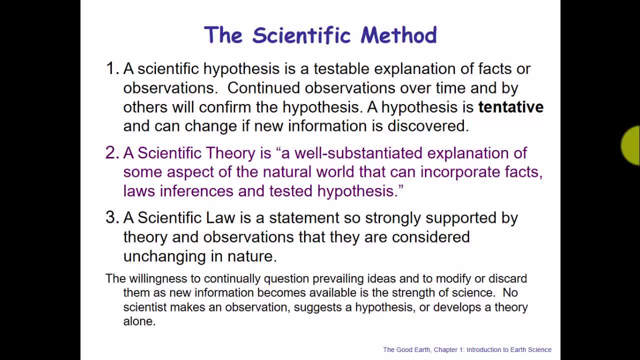 It's showing how good science built on observations over literally hundreds of years to come up with one theory after another theory, and now we have a scientific theory that is well-substantiated. Scientific law is something that is so strong and so rigid that we typically don't see new scientific laws. 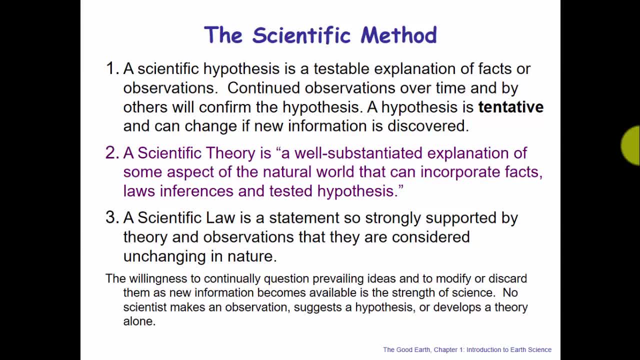 There have been lots of laws in the past, but this notion that a hypothesis and a theory has to be able to be changed if new information is discovered makes it more difficult to have a scientific law. But a scientific law is then a statement that is so strongly supported by theory and observations. 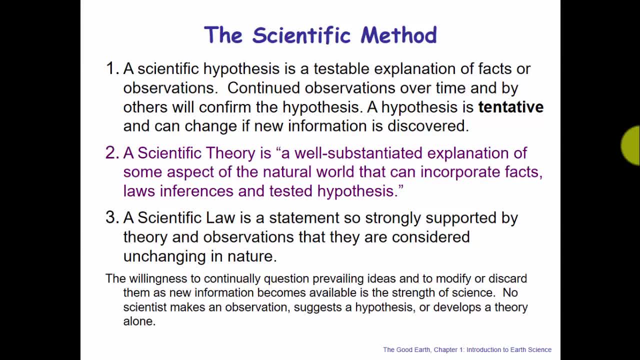 that they are considered unchanging in nature. And again, there are some things that we think are absolutely permanent. don't change. they'll always be this way. the sun will come up tomorrow. that would be a law. But if we had new data that came in? 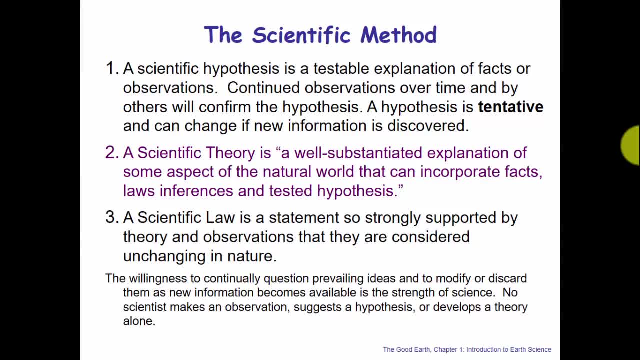 that was able to change the explanation or change the prediction, then that's where scientific laws may not hold up. But a scientific law is something that's so strongly supported that we think that it will always happen that way. So the willingness to continually question prevailing ideas, 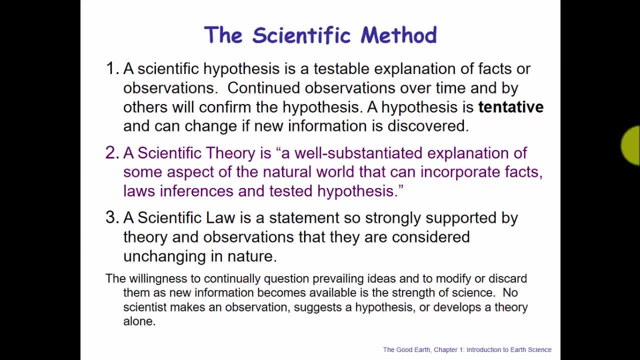 and to modify or discard them as new information becomes available is really the strength of science, This notion that if new information comes in, we've got to be able to get rid of, discard or at least change old ideas. And if you're not willing to change, 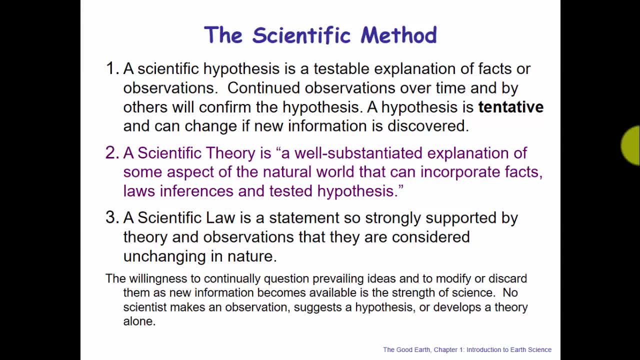 with new data, then you're not doing good science. No scientist makes an observation or suggests a hypothesis or develops a theory alone. This is all done by the entire scientific community, with different people testing hypotheses separately, testing ideas separately, bringing in data separately. 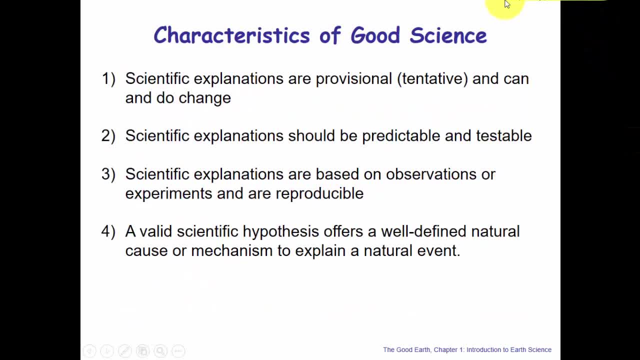 and all coming to the same conclusion. Now, I have used the term good science once or twice already, so what are the actual characteristics of good science? Scientific explanations are provisional, They're tentative. They can, they do and they should change. 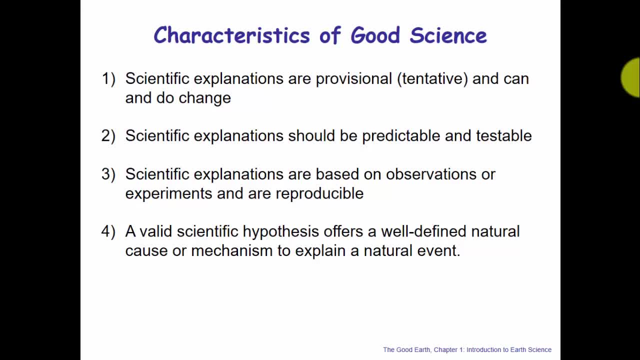 particularly when new information comes about. We've sort of harped on that a little bit now so that should be clear to you That if new information comes in, science has to be able to change, And if science can change it's provisional tentative, that's good science. 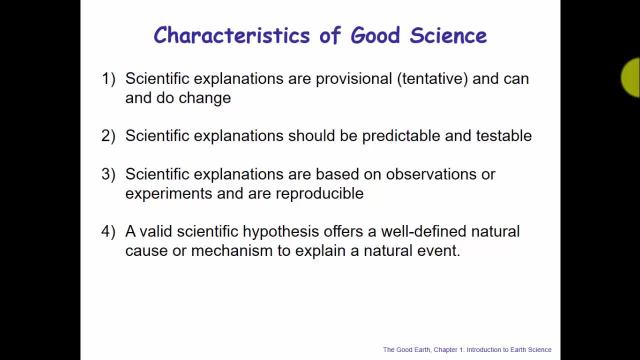 Scientific explanations should be predictable and testable. Again, you should be able to test one to the other. You should be able to set up a situation, model it whether physically or with a computer, or you should be able to run experiments in a lab. 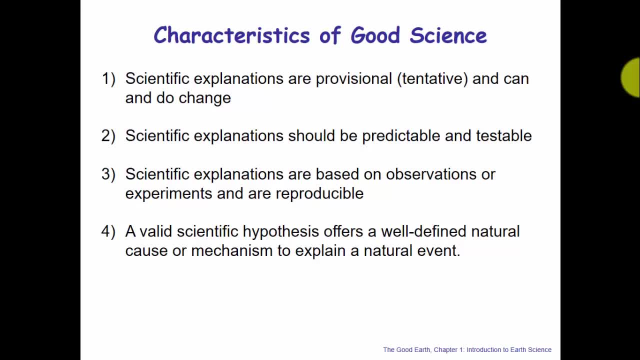 that test those scientific explanations. Scientific explanations are based on observations or experiments and therefore they have to be reproducible. If you do an experiment that proves that cold fusion is possible and economical, and so you go to claim that you can solve the world's energy problems, 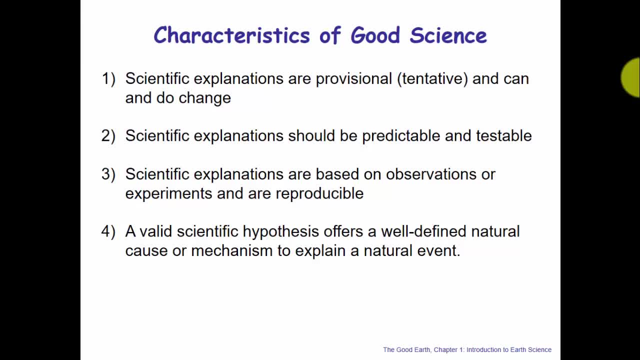 if that experiment is not reproducible by somebody else, then that is not good science, That's just an outlandish claim. And then valid scientific hypotheses have to offer that well-defined natural cause or mechanism to explain the natural event. So okay, volcanoes are a function of magma. 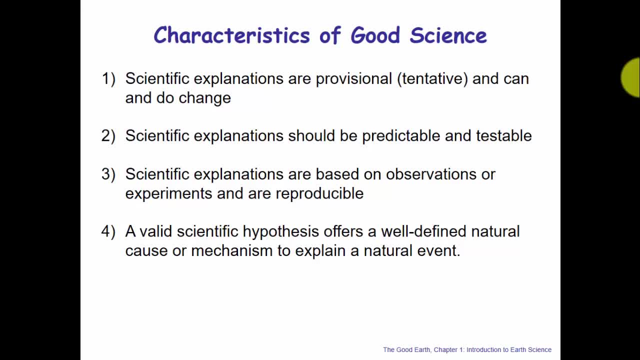 and the Earth's surface. so how did the magma get there? What's causing it to come up to the Earth? I mean, there's got to be an explanation or a mechanism, and if you don't have that mechanism in place, that's not good science. 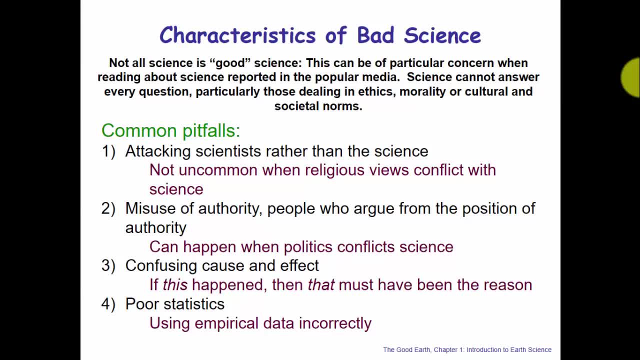 Not all science is good science, and this can, of course, be of particular concern when you're dealing about science as reported in the popular media. Science absolutely cannot answer every question. It can't deal with ethics, morality or culture or societal norms. 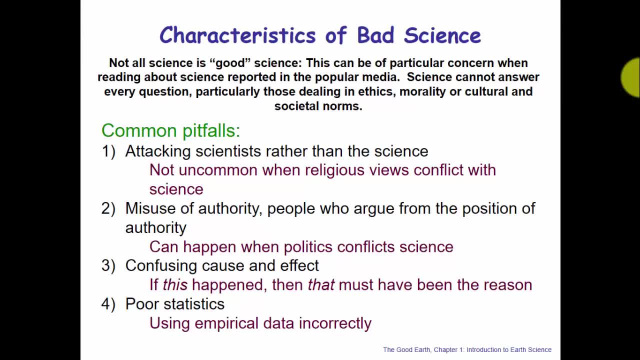 There are no experiments that can come up with theories or laws that control any of those things, But oftentimes people use science or attack science in order to advance their understanding of their own personal agenda. So the common pitfalls or the common characteristics of bad science include attacking the scientist. 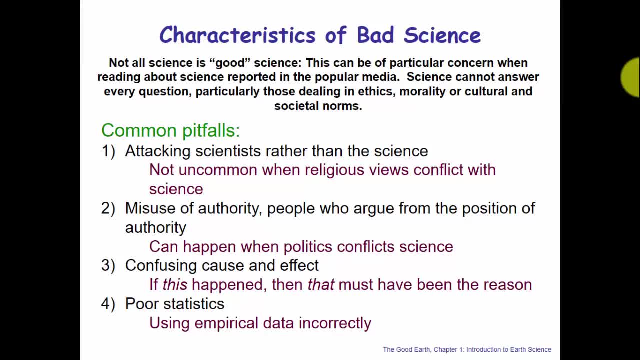 rather than the science, the misuse of authority, confusing cause and effect or just bad data, So attacking scientists rather than the science. this is a situation where individuals are attacked, made personal attacks on them, as opposed to the science that they're doing. 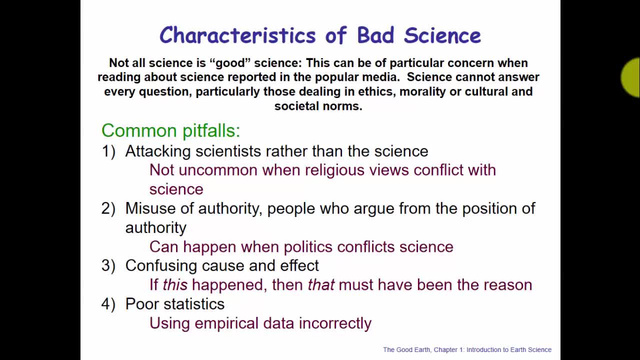 and not uncommon when religious views do conflict with science. The misuse of authority- and this is when people argue from the position of authority, and this often happens when politics conflicts with science. Somebody in high authority takes a position, that I'm in this position and therefore I'm right. 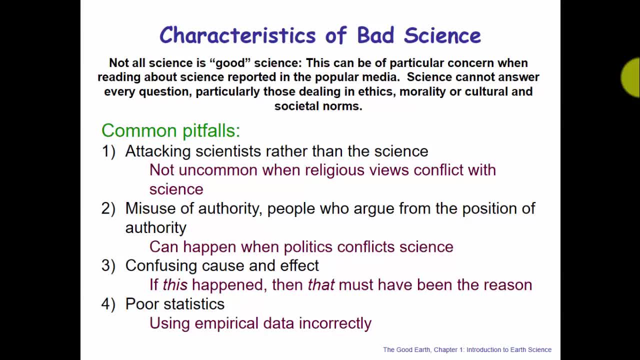 and they're not really considering the science. Confusing cause and effect: this notion that if this happened, then that must have been the reason, and that's not always the case. Sometimes the reason for occurrence is completely different. So, confusing cause and effect. 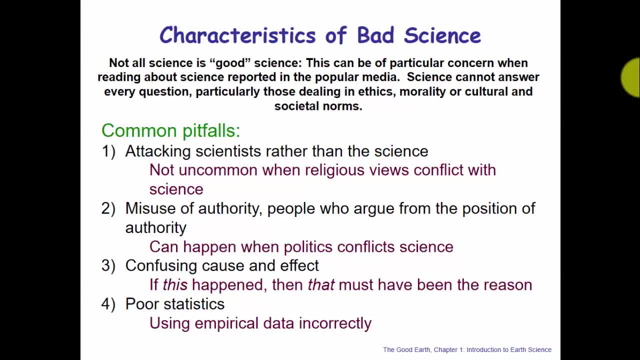 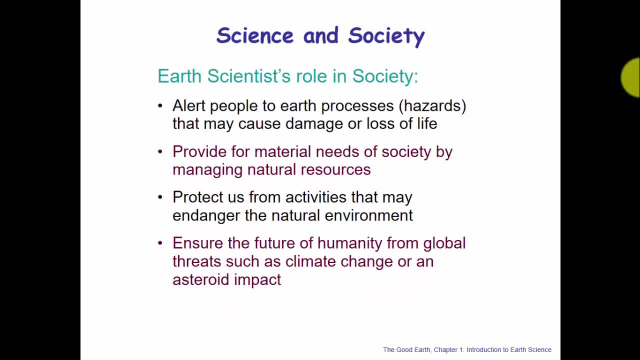 and also poor statistics, using bad data, empirical data incorrectly, just good data sometimes used incorrectly- all parts of characteristics of bad science. So what is society's responsibility to science and what is science's responsibility to society? It seems like an open-ended question. 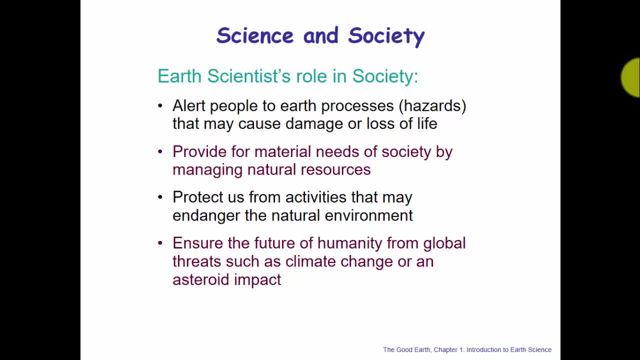 but when we're talking about the latter, there's actually some very specific points. Scientists and science is meant to alert people to the earth processes and, specifically, hazards that could possibly cause damage or loss of life. Science is also there to provide for material needs of society. 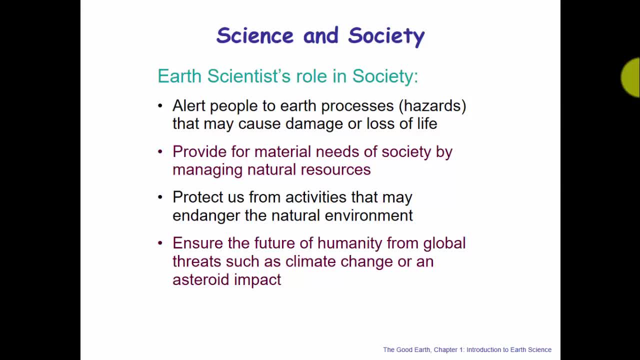 by managing natural resources. Science is there to protect us from our own activities that may endanger the natural environment, And science is there to ensure for the future of humanity from global threats such as climate change or near-earth objects, asteroid impacts, that type of thing. 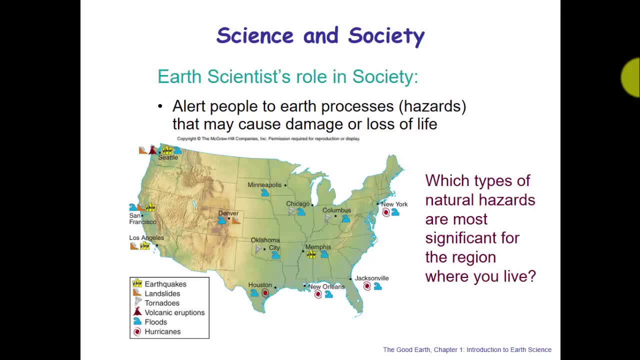 How do science and society interact Well, earth scientists' role in society is to alert people to the earth processes or hazards that may cause damage or loss of life. So which type of natural hazards are most significant in the region where you live? So you can see Florida here with Jacksonville. 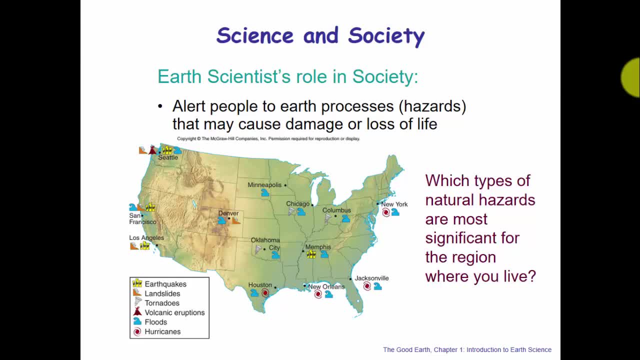 and New Orleans as well, The hurricane and potentially flooding. in our case, flooding is going to be coastal flooding, which is likely to be brought on by a tornado, which is likely to be brought on by a hurricane, which is likely to be brought on by a tornado. 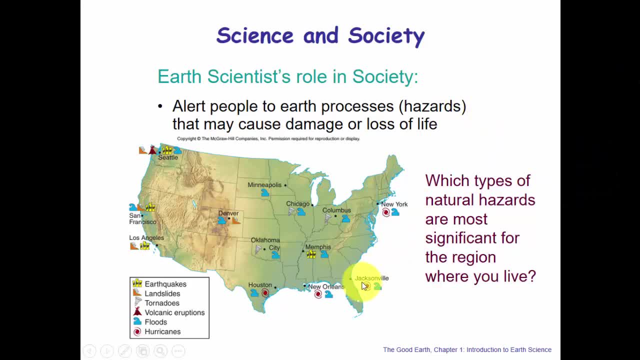 which is likely to be brought on by a tropical storm. But in all different parts of the country there are different hazards that scientists are responsible for letting people know about. For instance, you know if you live in Seattle or San Francisco or Los Angeles. 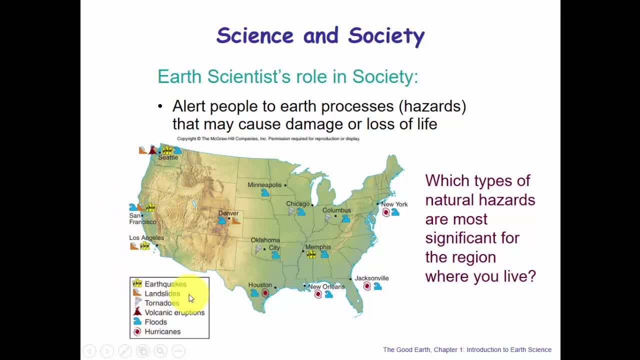 you're fairly aware already that earthquakes are a problem, But did you know if you were in Memphis earthquakes can be an issue as well? The types of things that earth scientists are responsible to let people know about In terms of alerting people to earth's processes. 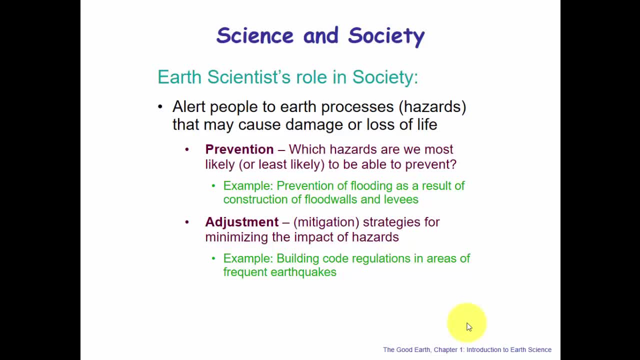 in terms of hazards that may cause damage or loss of life, So great you let somebody know. What else can a scientist do? Well, scientists work toward prevention, and also toward mitigation or adjustment, as it's listed on the slide. Prevention, of course, is in which hazards 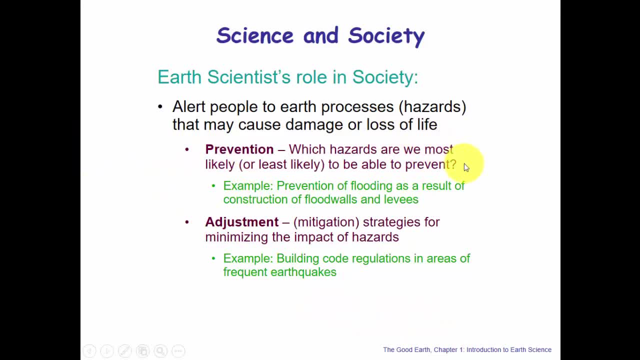 are we most likely, or at least possibly able to prevent? Flooding is one of those things. Flooding can be prevented through flood walls or levees. Hurricanes probably can't be prevented, Tornadoes likely not, But science can have strategies for minimizing the impacts of those hazards. 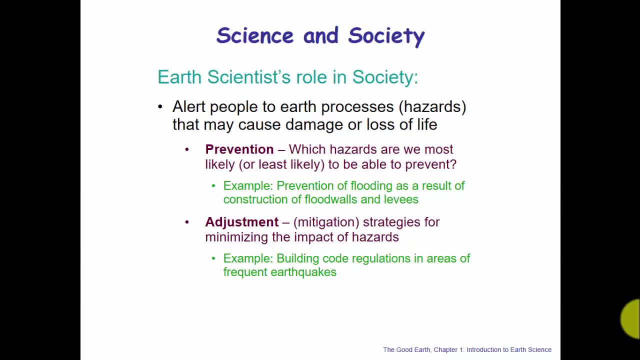 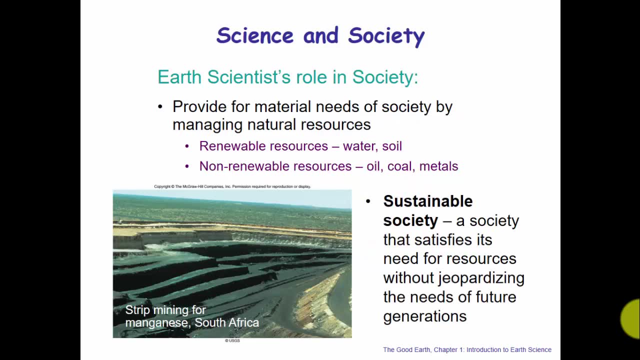 like building codes in areas of frequent earthquakes, That's, adjustments made by science or mitigation strategies proposed by scientists. Earth scientists should also help to provide for material needs of society by managing natural resources, including renewable resources such as water and soil. Also non-renewable resources such as oil, coal and metals. 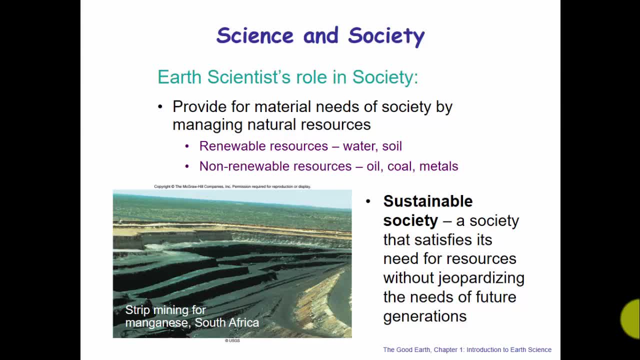 And earth scientists typically want to work toward a sustainable society, a society that satisfies its need for resources without jeopardizing the needs of future generations. Do we have a sustainable society now? Are we capable of becoming a sustainable society in the future? And this notion of sustainable or sustainability? 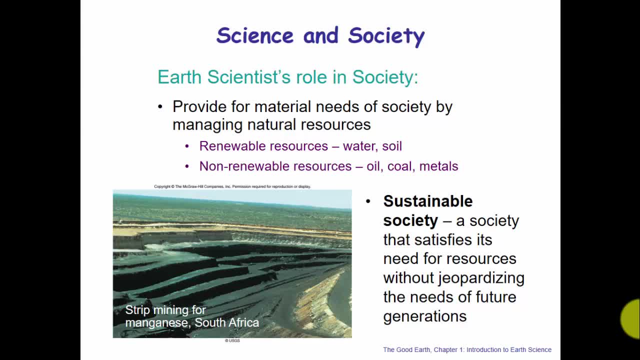 is something that, as you're looking toward your coursework in the future and what you might want to study further and perhaps even make a career out of, sustainability is a word that we're finding in very high-level positions now in major corporations that did not exist 10 years ago. 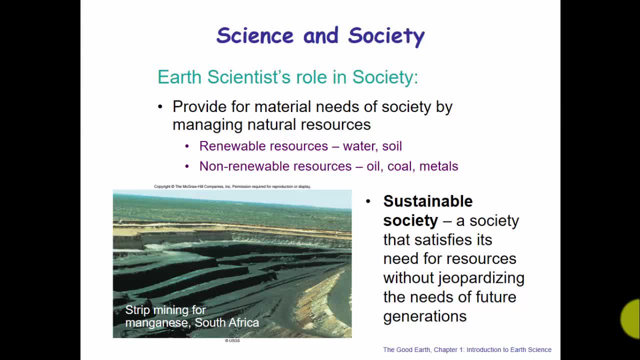 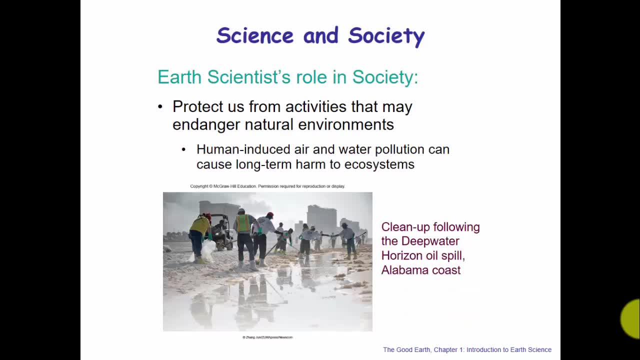 And so sustainability and the science of sustainability is a great way, in the future, to make a living. Earth scientists also want to protect us from activities that may endanger natural environments, So earth scientists should be working toward preventing human-induced air and water pollution that can cause long-term harmful effects to ecosystems. 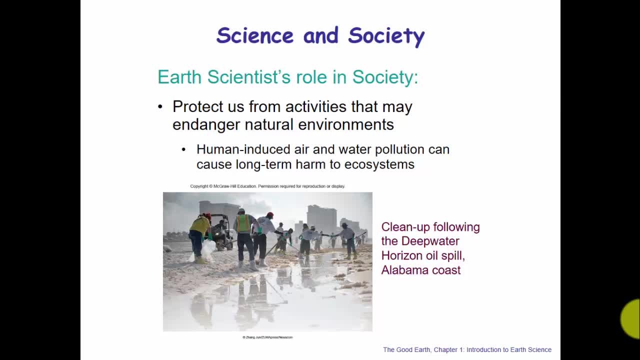 It should provide methods in the science to help clean up following major catastrophes like Deepwater Horizon, the oil spill along the Alabama coastline. So that's another role of the earth scientists in society is the protection of society from activities that may endanger natural resources. 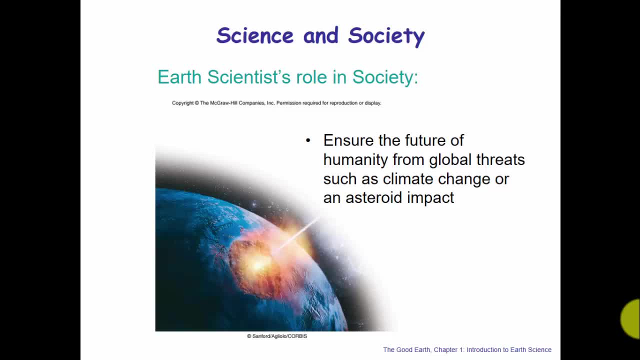 In terms of the role that earth scientists play in society. lastly- and maybe this is a bit of a larger scale, but lastly- earth scientists are there to help ensure the future of humanity from global threats. Now, the two main global threats: 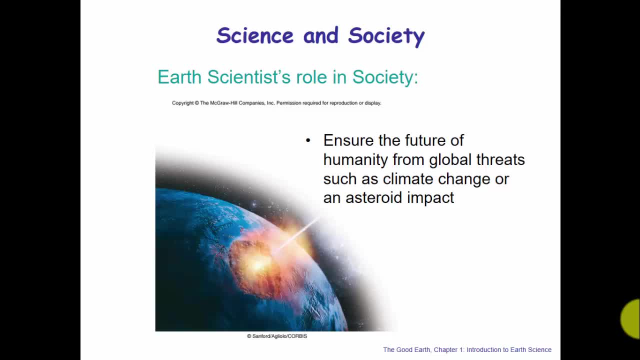 we're talking about these days, and what we talk a lot about in this course, are climate change, of course, but also things like near-earth objects and asteroid impacts, And earth scientists are looking at both of these situations to try and determine can we prevent them? 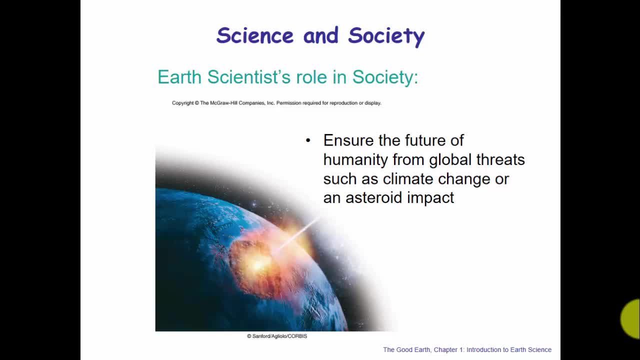 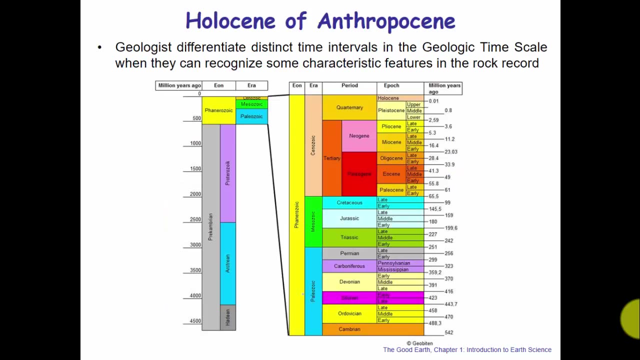 or if we can't, can we at least mitigate the impact? So, as you can see, the earth scientists not just about rocks, but has a major role in society, in helping society be a better place for all of us. So we'll wrap up chapter one. 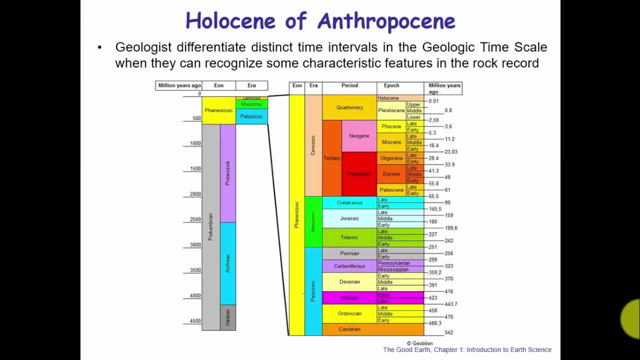 and an introduction into earth science, with a look at where humans, where homo sapiens, stand in the history of earth and what has been the impact of this species- homo sapiens- on earth. So, speaking of theories, one theory that had to change a great deal. 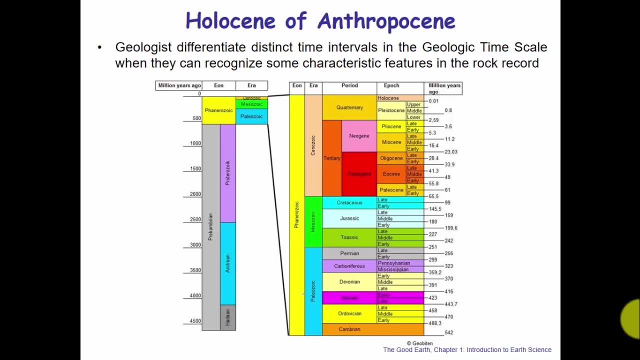 as new data came to light, was the theory as to how old the earth is and how did the earth get here. Geologists or scientists think of the time that earth has been in existence on a scale known as the geologic time scale And the geologic time scale. 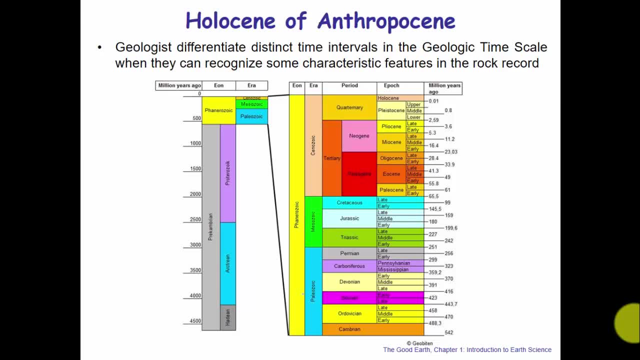 is the scale of distinct time intervals from right now all the way back to the formation of the planet, And they recognize some of those distinct time intervals based on classic features that they find in the rock record. We can go to the Grand Canyon, and because the Grand Canyon 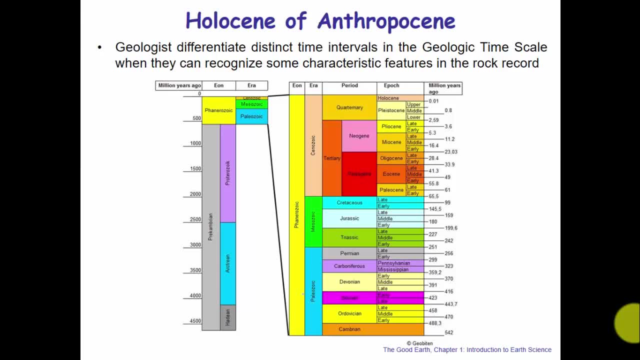 or the whole Colorado Plateau was uplifted, the whole massive region of the Four Corners area uplifted by some tectonic activity, and then the Colorado River dug down into that uplifted rock and exposed all these different layers from the Neogene to the Paleocene. 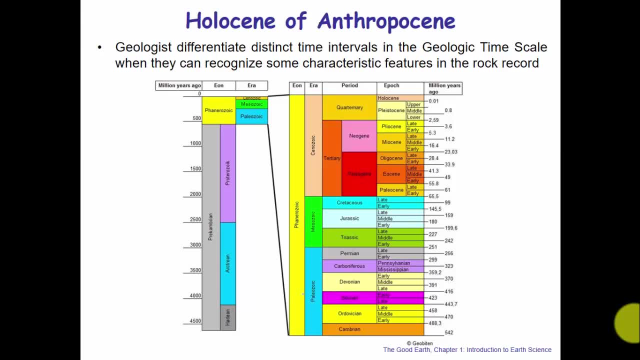 to the Cretaceous, down to the Devonian and the Orvician, all the way down to the Cambrian. We can see these distinct time intervals in the rock record of the geologic time scale, Now on the left, in millions of years. 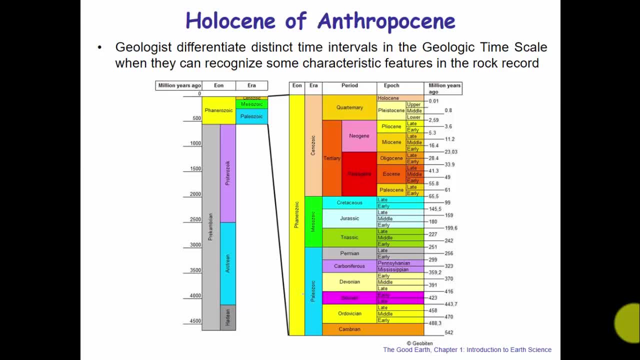 you go down that column and you get all the way back to 4,500 million years. Not 4 million years, not 45 million years, not 400 million years, not 50 million years, but 4,500 million years. 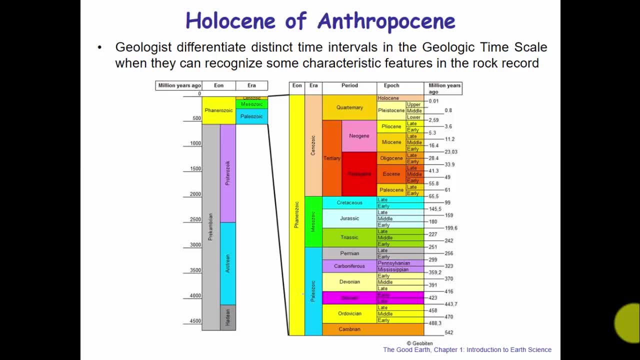 or 4.5 billion years ago, And scientists believe that the Earth was formed some 4.5 billion years ago And in the very beginning. very little exists in the rock record known as the Hayden period and really right on through the protozoic period. 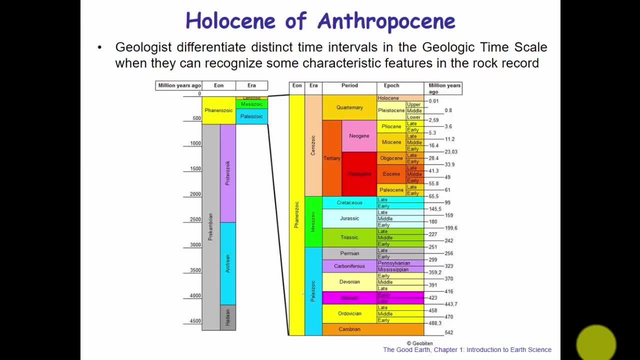 which takes us all the way up almost 4,000 of those 4,500 million years. So we really don't begin to see things in the rock record until we get to that period of about 500 million years ago, the Phanerozoic. 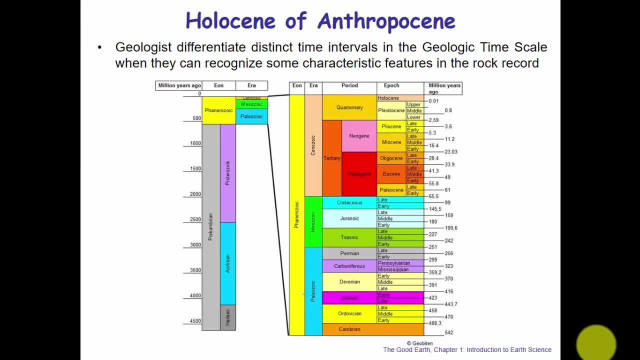 We're talking about the Paleozoic and the Mesozoic and the Cenozoic, And from that we start to see things in the rock record. And the point of this is, first off, to try and give you your very first peek. 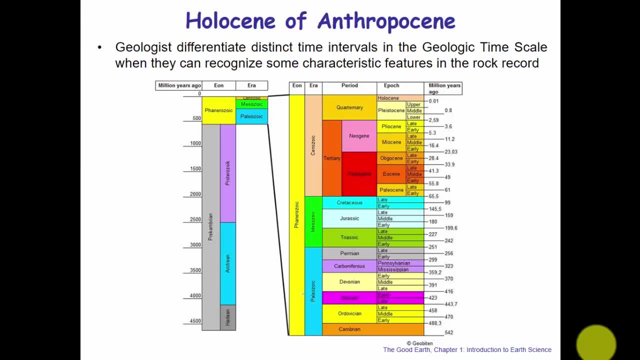 at geologic time and just how large it is, and then some idea how the eons and the eras and the periods and the epochs have been broken down: The Paleozoic broken down into the Cambrian, Orvician, Silurian. 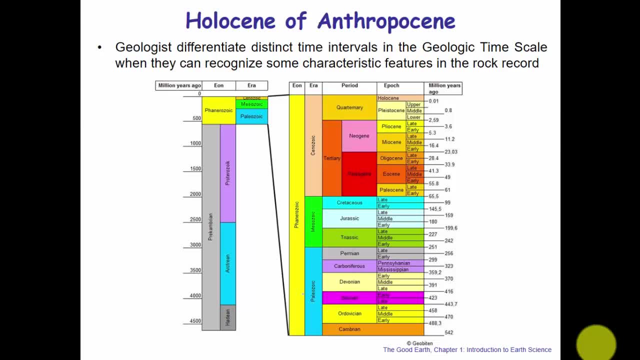 Devonian and so on and so on. And then let's say, the Carboniferous period is the Mississippian and the Pennsylvanian, and that's when coal was being formed. So all these different periods and epochs and eras, and even eons. 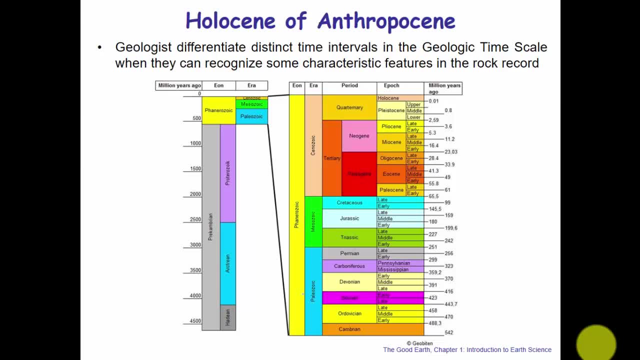 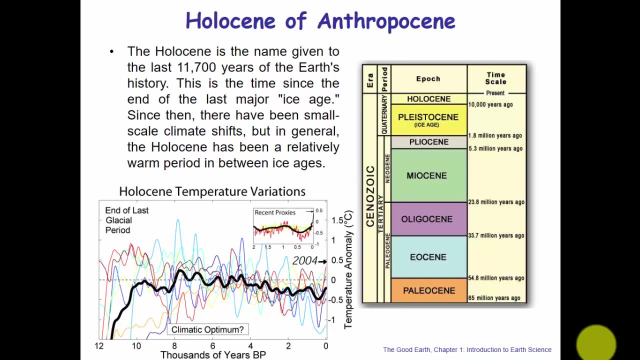 are all distinct in the rock record And that's your geologic time record. So if we go all the way up to the Cenozoic era and then into what's known as the Quaternary period, we see the Paleocene. 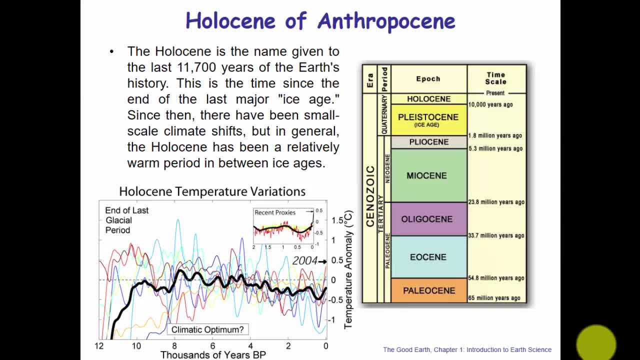 the Eocene on up to the Pleistocene, that's the Ice Age and the Holocene. So the Holocene is the epic that is given to the last 11,700 years of the Earth's history And this 11,000 year period. 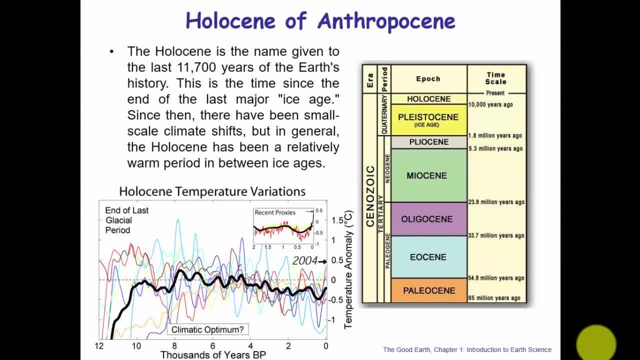 is the time since the end of the last major Ice Age, So it was during the Pleistocene period that the last major Ice Age occurred Now, since then, there have been small climatic shifts. We've had some warmer periods, some cooler periods. 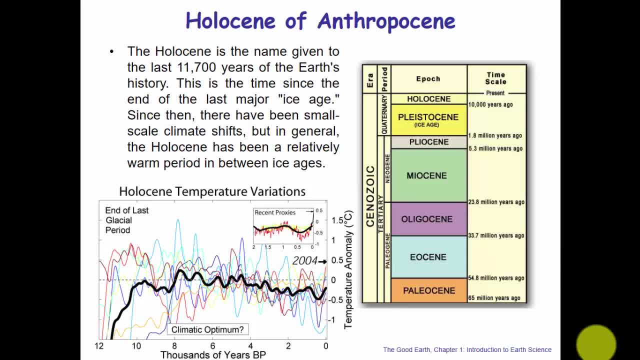 but generally in the Holocene it's been a relatively warm period. That's what's referred to as interglacial period between glaciations, And so the epic that we are in right now 10,000, 11,700 years ago. 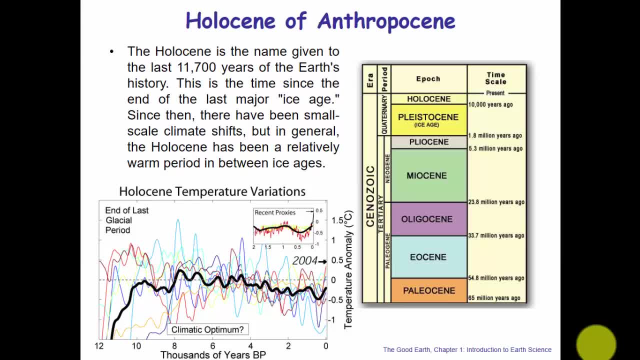 until present is known as the Holocene, And scientists- or at least some scientists- are beginning to think that we need to put a new line, a new change in the record and have a new epic and have the Holocene be something that's in the past. 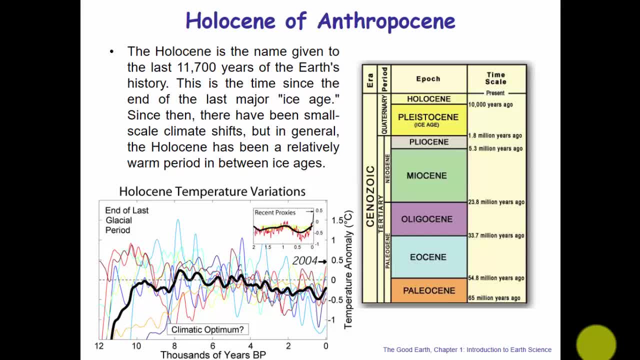 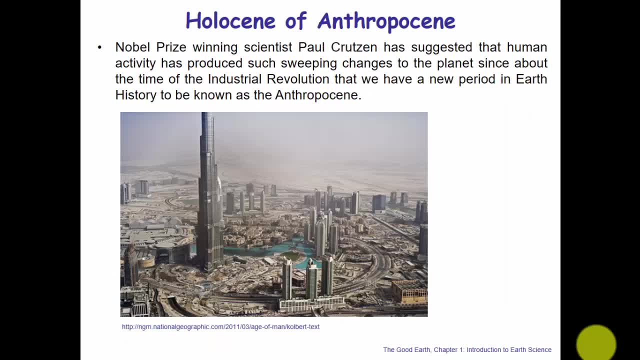 and a new epic based on the impact that humans- almost sapiens- have had in the rock record. So scientists like Nobel Prize winning scientist Paul Crutzen has suggested that human activity has produced such a sweeping change to the Earth itself since about the time. 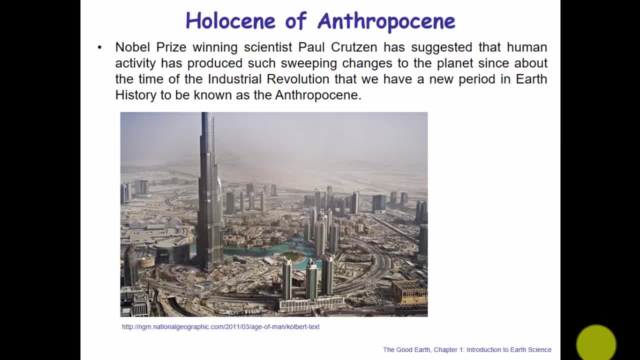 of the Industrial Revolution, that we have a new period now in Earth that would be known as the Anthropocene, And so the suggestion, that is, if the Earth is around another four and a half billion years, that geologists looking at the rock record would see the places seen.